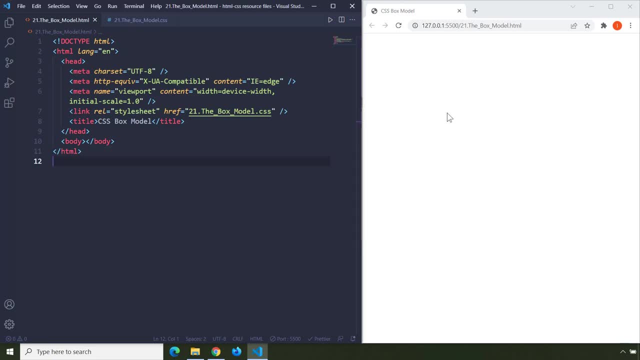 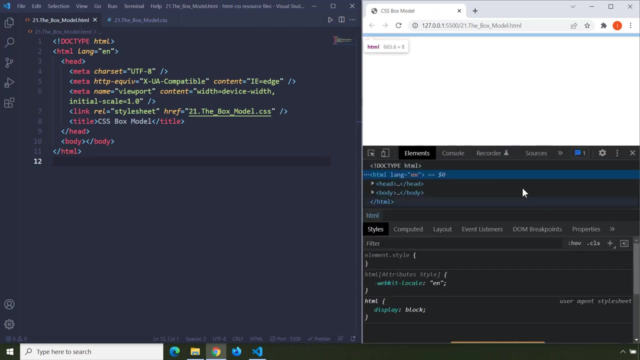 the bat so we can understand CSS way better. Now, here we have our HTML, here we have an empty CSS file And here I've opened the CSS box- modelhtml file. I'm going to go ahead and I'm going to right click and I'm going to say: inspect. When you inspect and when the Chrome window is small. 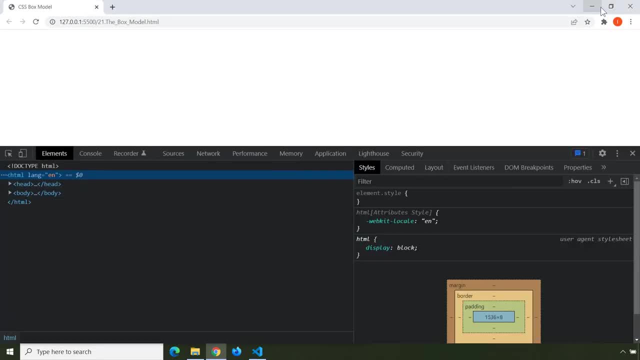 you're going to see CSS HTML on top and CSS in the bottom. But if you go full screen on this Chrome, on the left side, we're going to see HTML. on the right side, we're going to see CSS. I'm going to. 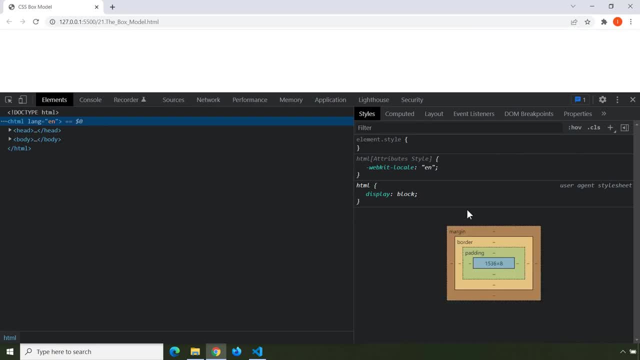 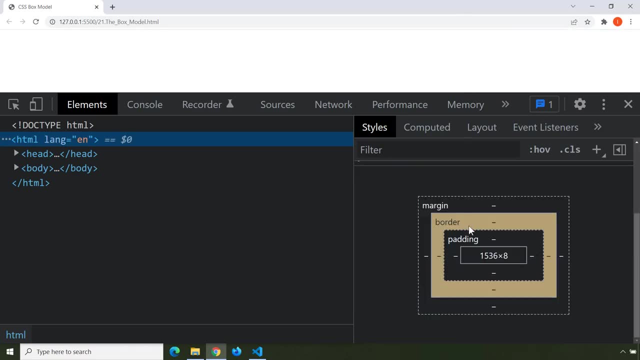 bring this up, This representation on the bottom right corner. I'm going to zoom in. This is the CSS box model. There we go. So this is one of the most important and fundamental concepts in CSS And if you want to master CSS, 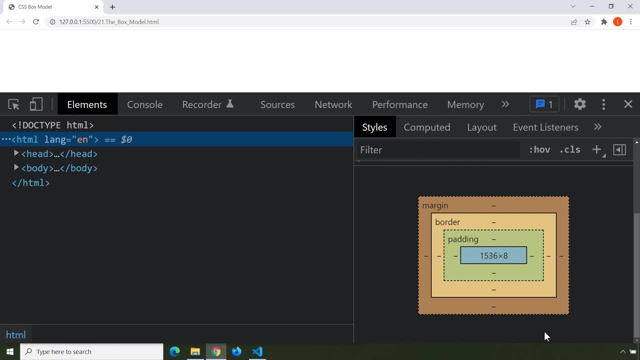 you need to learn this first. Now, CSS box model says: everything in CSS is a box. Excuse me. So when we have boxes in CSS, what does that actually mean? What does this sentence mean? That everything in CSS is box? I mean, CSS is nothing without HTML, And if we don't, 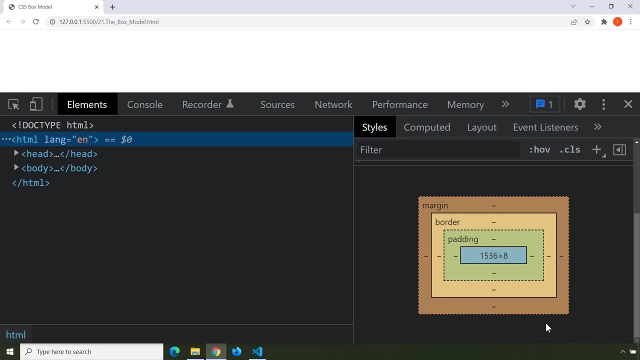 have any HTML. we don't have any CSS either. So what it? what it actually means is that every HTML element is considered to be a box in CSS, So it doesn't matter what that HTML element is, even if it is the HTML root element, the body element, the head element. h1 paragraph. 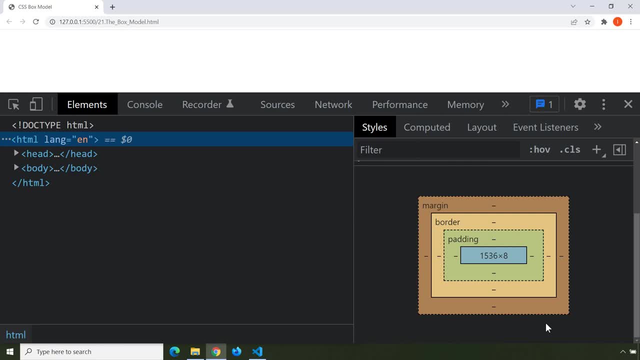 buttons, images doesn't really matter, As long as it is in the realm of HTML. it is, it is considered to be an HTML element, But when it crosses over to the realm of CSS, CSS considers that element to be a box. Now, when it is a box, it is going to contain different properties, different sections. 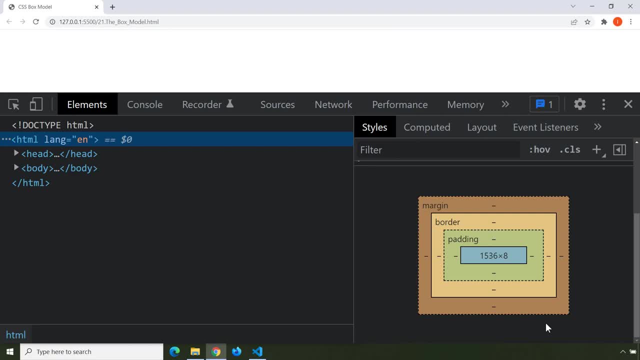 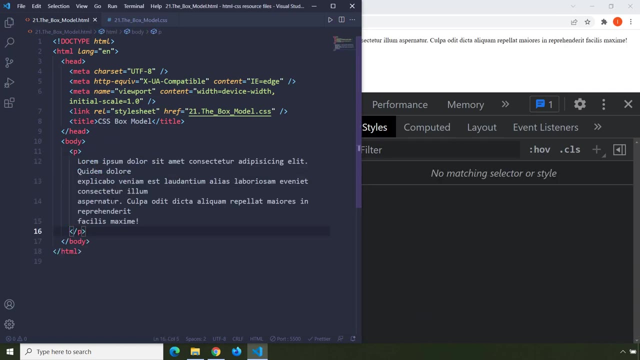 different components. Each box consists of four major sections, So the first one is the content within that box. So let's take a look at each of them one by one. I'm going to create an HTML element, And when this HTML element is crossed into the world of CSS, 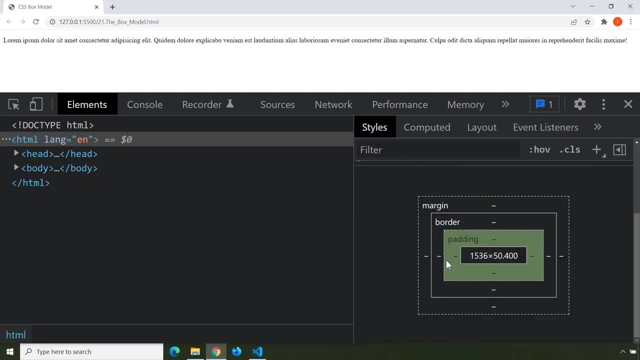 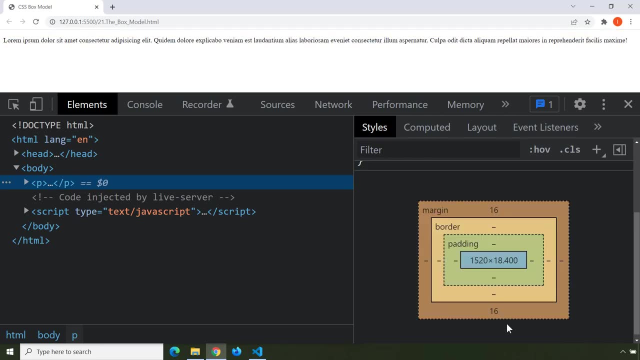 it is going to become a box, to keep that in mind. So let's go ahead and let's select it here. So this is our paragraph. There we go. Now let's talk about this box model. we are going to cover each individual part or component of this box model, like padded, something like that. So what we're? going to do is we're going to anchor it to a description of this box. what we are going to do is we're going to create a PDF file which is a little bit more complicated. we're going to create a PDF file which is a little bit more complicated. we're going to create a PDF file which is a little bit more. 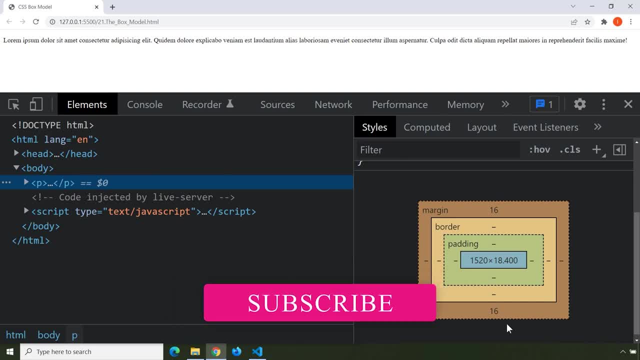 border and margin in our upcoming lectures. for now, this is just a general overview of that. so what do we have here now? every HTML element- again when it crosses over to the world of CSS- is a box. each box consists of four major parts. the first one is the content of that box. there we go, so 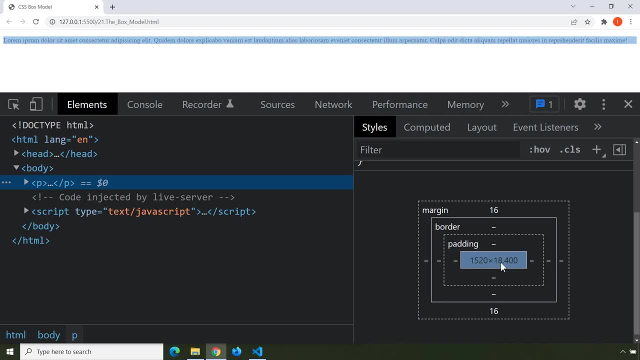 this: the inner, the most inner part or rectangle, is the content and when you hover on it, only the content of that box will be highlighted. as you can see in our web page, it is highlighted and it has some sort of blue overly. it is not a background, it is an overlay and it shows the 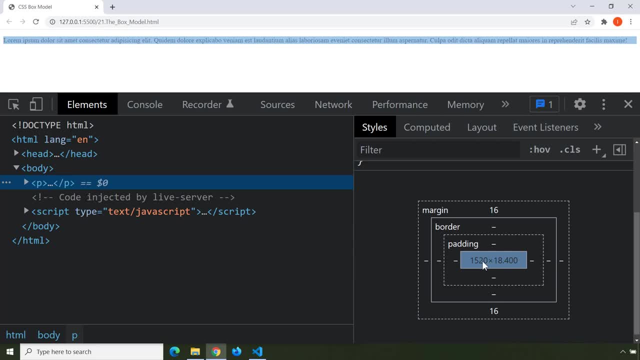 dimensions of that content. the first value is the width, or the horizontal dimension, and the second one is the height or the vertical dimension, so it is 1520. it means that there are 1500 and 20 pixels within that fiber gal switches. only a single file in the title. And when we also cooking us fierce. 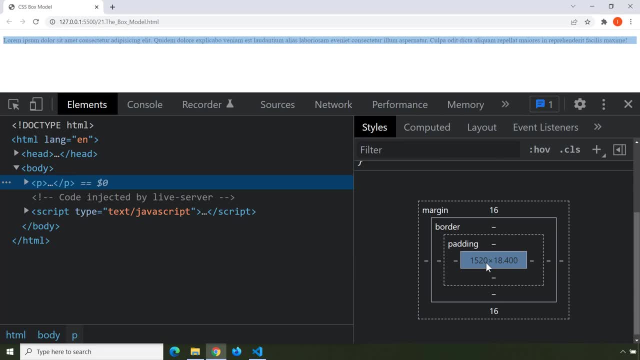 help. I provided a little bit of examples in process, so it goes like this: if you want, you can. the horizontal dimension of this box, the content of this box, not this box, this general thing, this entire thing is the box, But this is the dimensions of the, the content of the box, And. 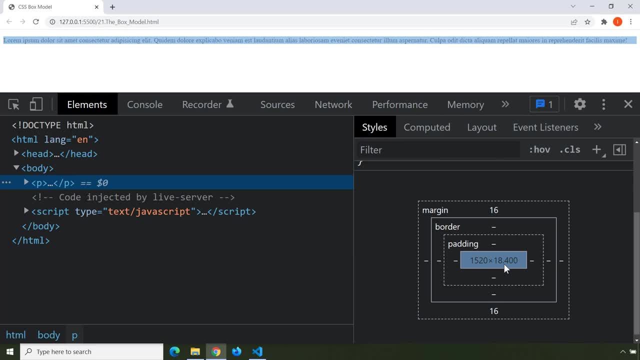 there are 18.4 pixels in the height or vertical dimension of this, the content of this box. These are very technical. If you understand this, then you will have understood the entire CSS. So after that, we have padding. we don't have any padding. That's why you can see there is like 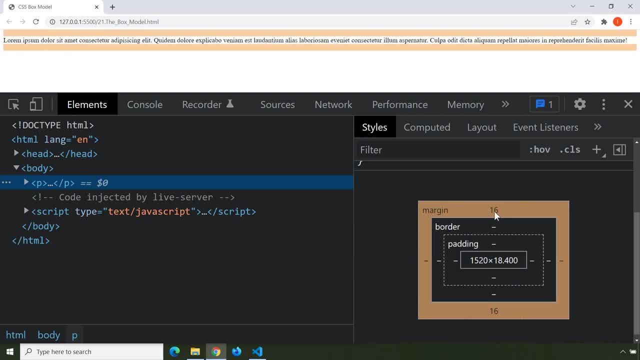 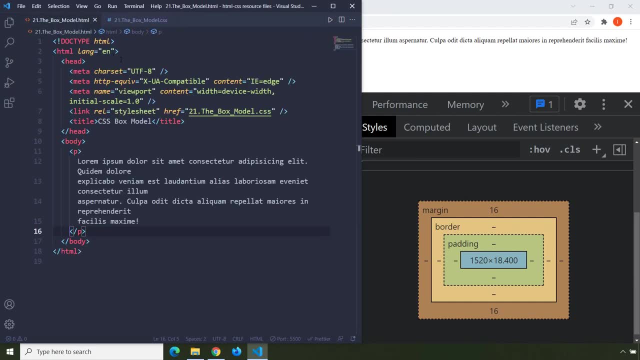 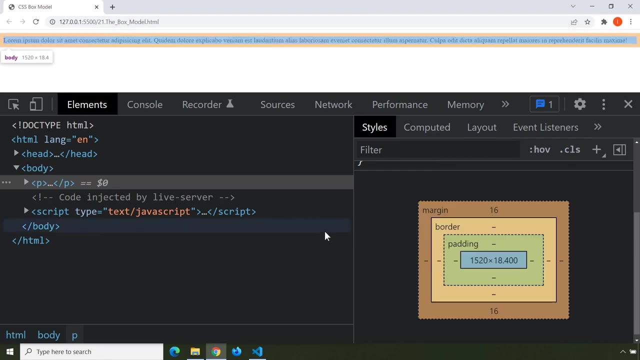 hyphens there, After that we have borders And after that we have margins. Now, we have not applied any styles on this paragraph. you can see that this style is empty. it is connected to this file, So where does these? Where did these two values they come from? We have talked about